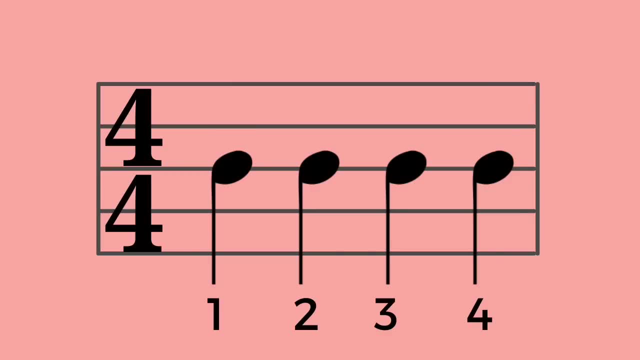 1,, 2,, 3, 4.. Now I want you to try it. Ready, get set, go Nice job. Now here's a measure of 4 quarter rests. When you count these, you can either leave it silent or say: 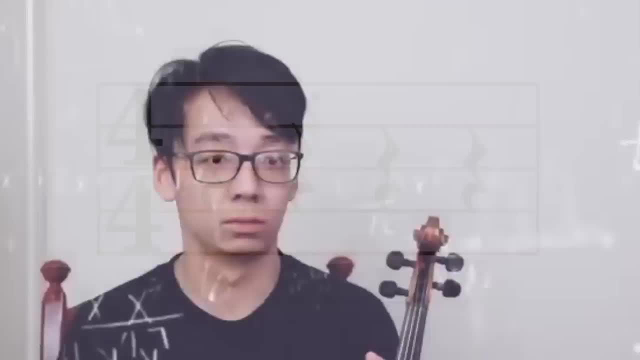 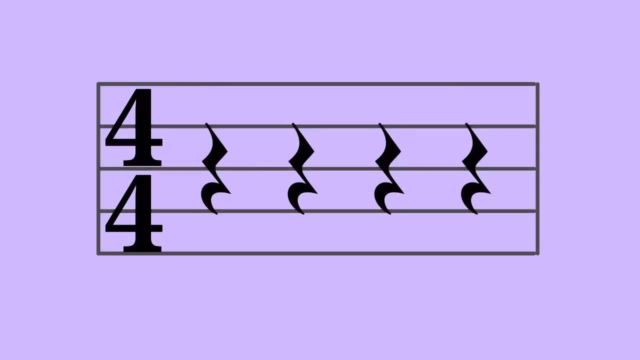 I recommend shh because it'll teach your brain to recognize rests actively, which, in turn, will lead you to developing a better sense of rhythm. 4 quarter rests sound like this. Now it's your turn. Ready, get set, go. 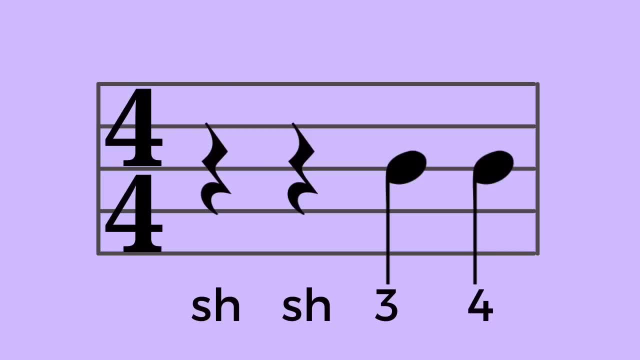 Awesome job. You can create all kinds of different rhythms simply by switching out the rests and notes. However, this is a very simple way to do it. The number is always going to be in the same place. For example, this last note is always going to be counted as 4. 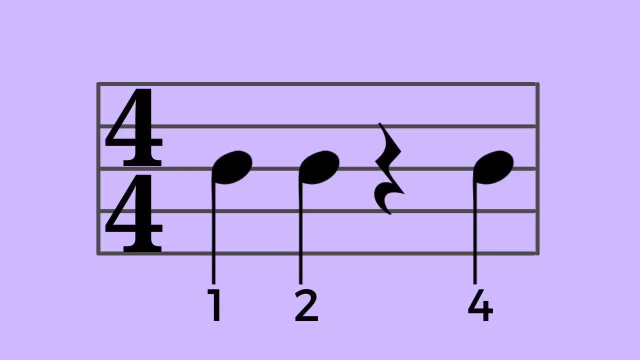 because it's the 4th beat in the measure. It's not 3, because the 3rd beat is right here. You just say shh, because it's covered by a rest. Oh hey, would you look at the time. It's drill time. 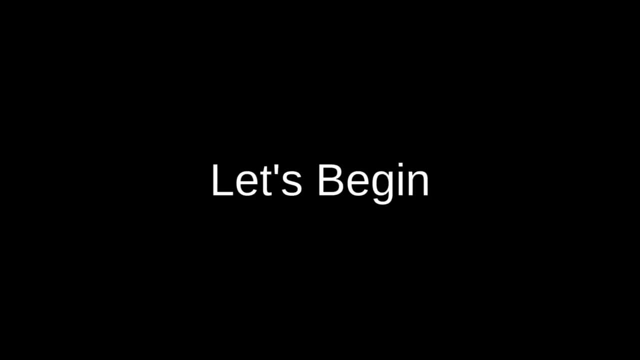 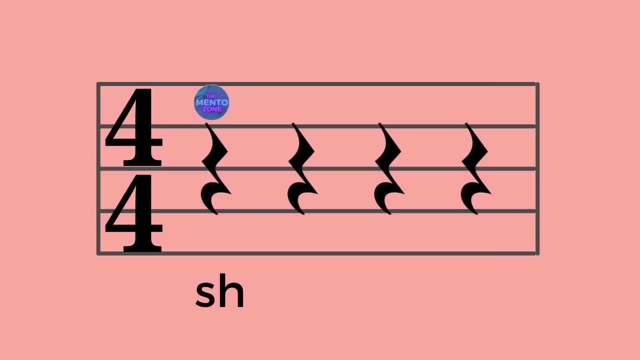 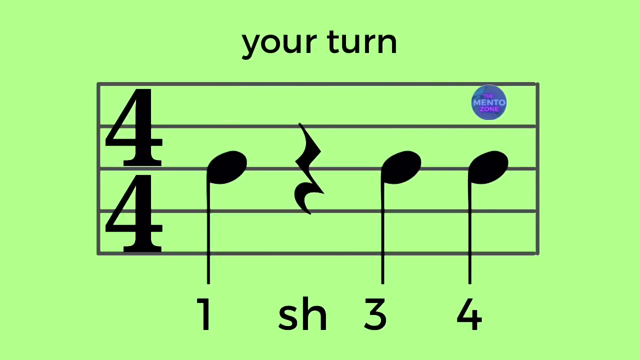 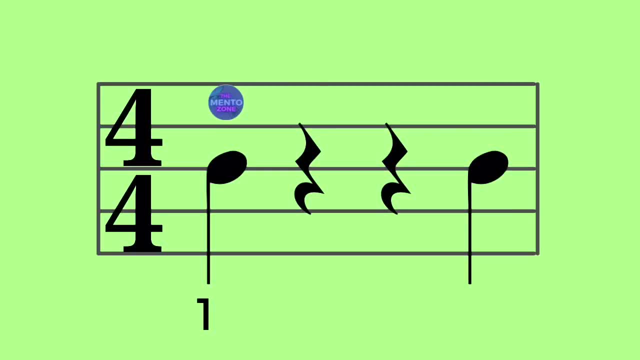 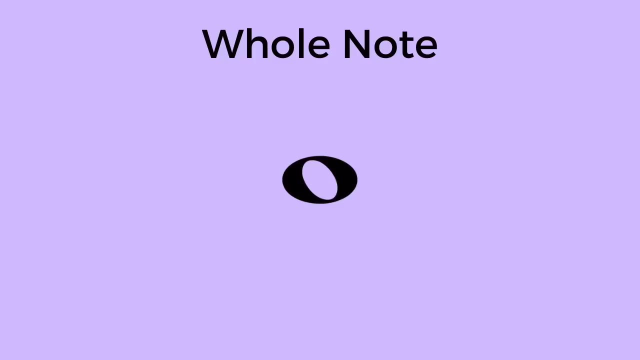 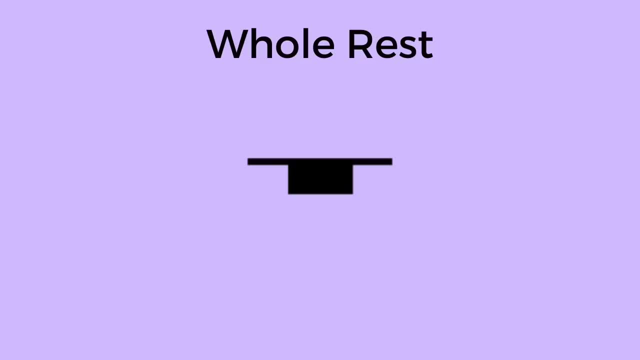 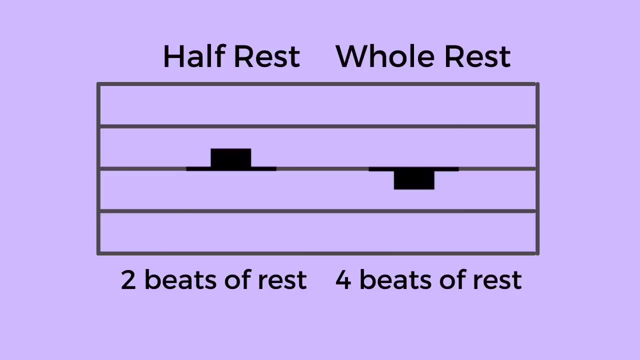 This is a half rest, It's worth two beats of rest. And this is a whole rest: It's worth four beats of rest. Now how do we count these? Let's start with the rests. These are pretty simple. You just say shh on every beat. 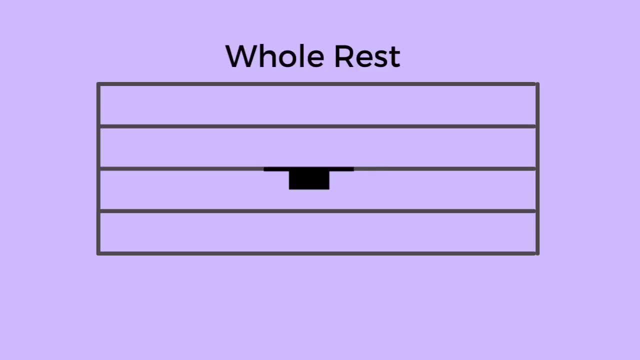 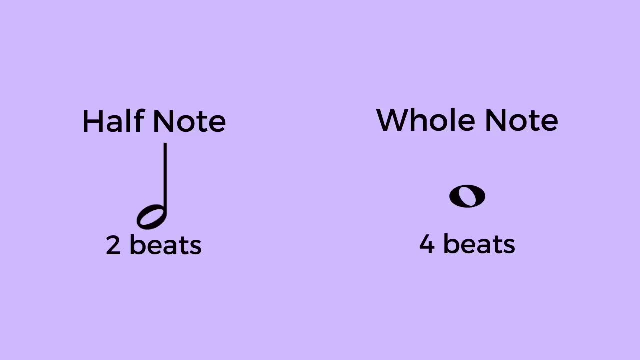 So your half rests are counted shh shh And your whole rests are counted shh shh, shh shh. The notes are a bit more challenging and there are lots of different ways to count them. I think the best method is you start on the number and then you bounce your voice for 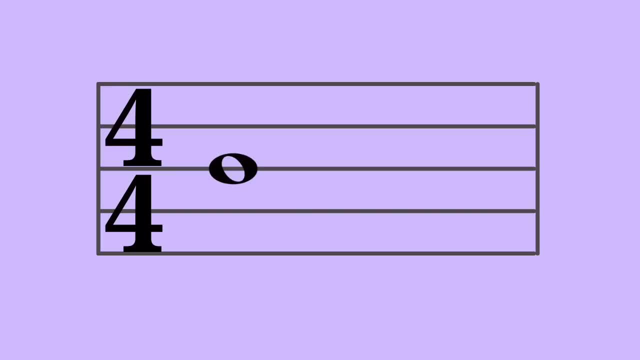 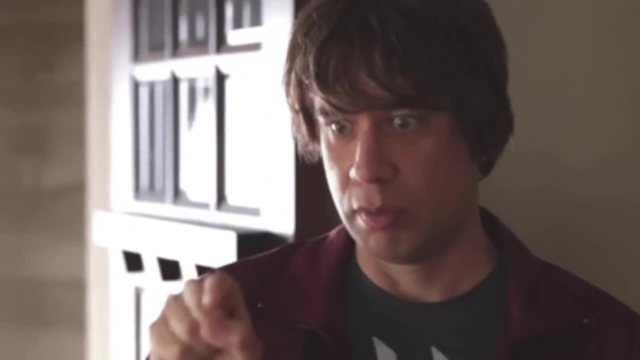 every following beat the note is held to. For example, the whole note would be counted like this one, Like saying shh on the rest. Bouncing your voice helps you think about held notes actively and helps you develop your internal pulse, which is extremely important to have in music. 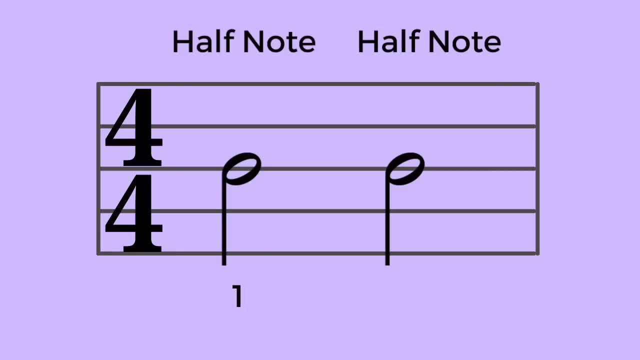 Two half notes would be counted like this: one three. Notice that beats two and four are contained within these two half notes. This is why we're skipping over them. And hey, would you look at the time again? It's another drill time. 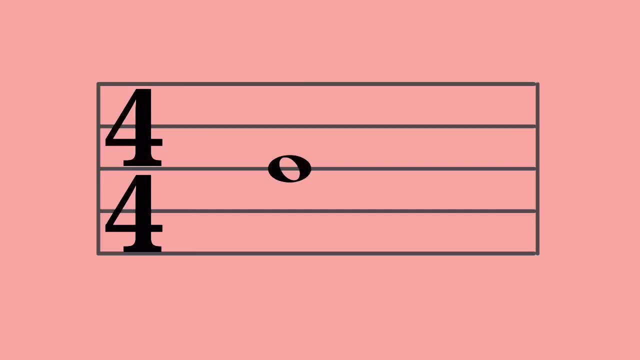 Same as before. First I go, then you repeat: One shh shh, shh, shh, One, three. One shh shh, shh, shh, Three. 1, 3, 4. 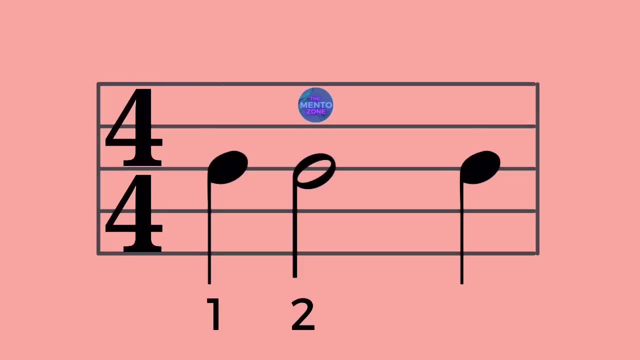 1, 2, 4. 1, shh 3. 1, shh 4 shh. 2, 4 shh. 3, 4 shh 2, shh shh. 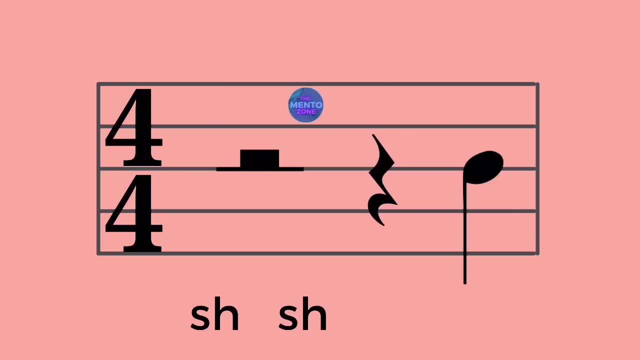 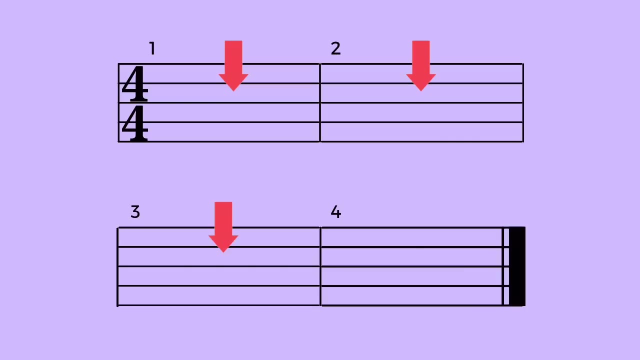 shh, shh, shh 4. Okay, one measure of call and response is easy, but what's actually more difficult is counting the rhythms correctly with multiple measures of music. Here are four measures of rhythm. Look at it, figure it out in your brain. 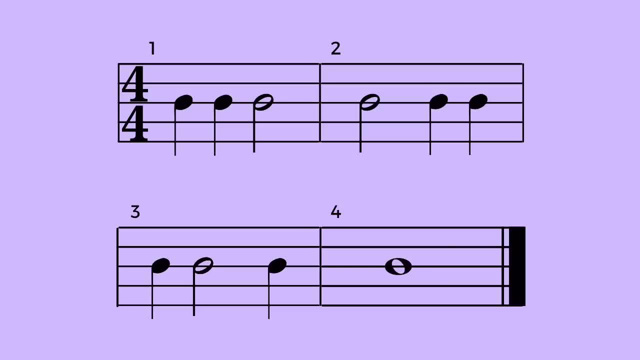 You're going to try it first, then we do it together so you can tell if you did it right. Prepare yourself: 1,, 2, ready go. Okay, let's do it together. 1,, 2, ready go. 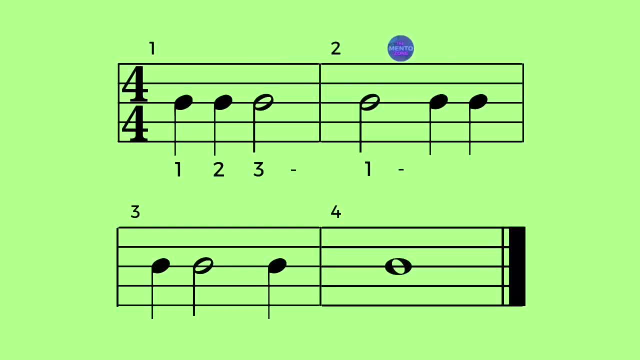 1, 2, 3, 1, 3, 4. 1, 2, 4, 1, 2, 3, 4. 1, 2, 3, 4, 1.. Did you do it correctly? 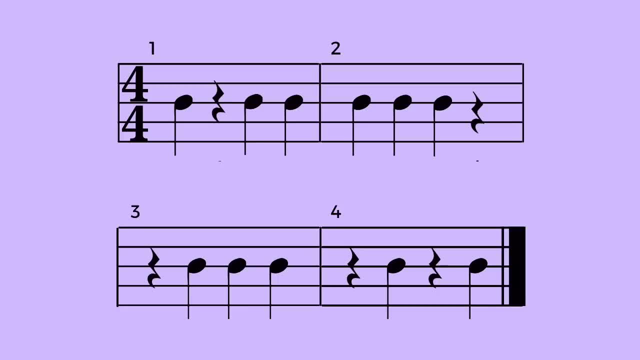 If so, let's move on. Next example: Pause the video if you need to take a look at it and, when you're ready, give it your best shot. 1,, 2, ready. go Alright now, together with me. 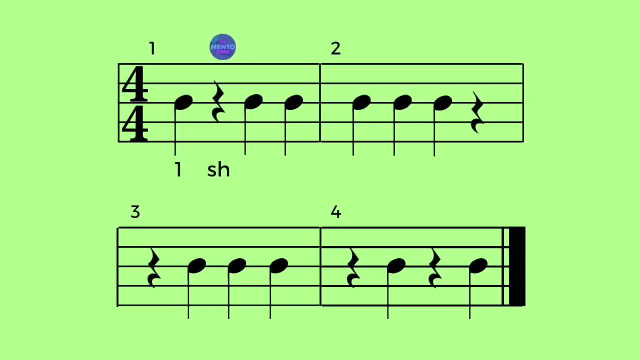 1, 2, ready go. 1, shh 3, 4, 4.. 1,, 2, 3, shh, shh. 2, 3, 4, shh, 2, shh, 4.. Next example: When you think you got it. 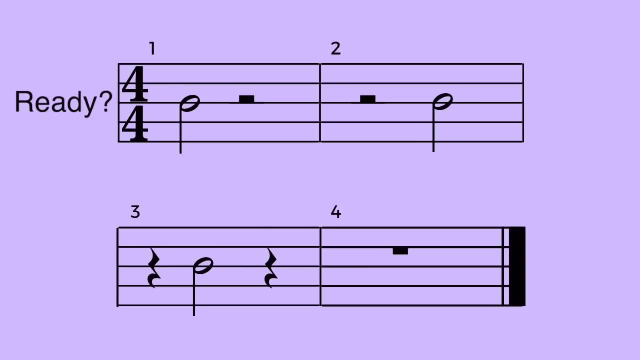 give it a shot: 1,, 2, ready go. And now with me: 1,, 2, ready go. 1,, 3,, 2, ready go. Next example: Take a look: 1,, 2, ready go. Alright, now together with me. 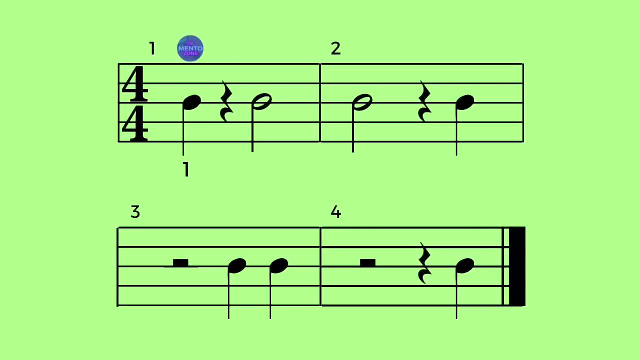 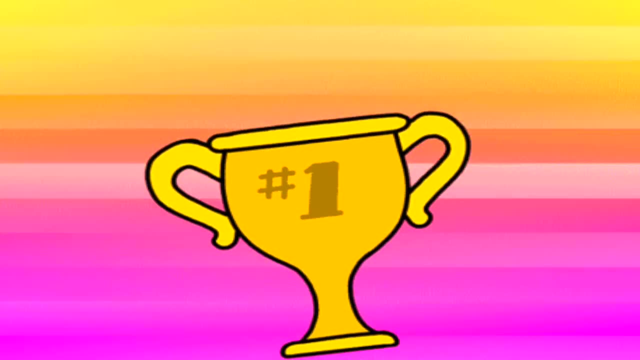 1, 2, ready go. 1, shh 3, 1, shh 4, shh shh 3, 4, shh shh 4.. Did you do all that correctly? If so, congratulations. You now know the basics.